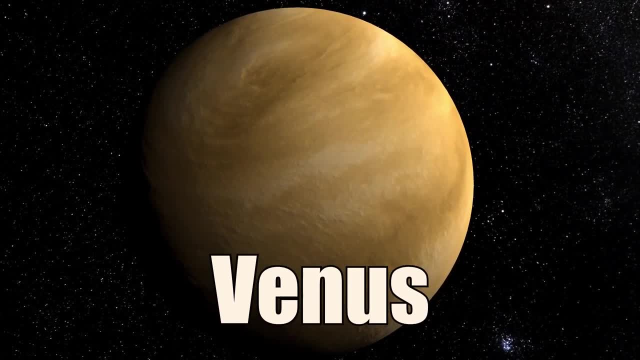 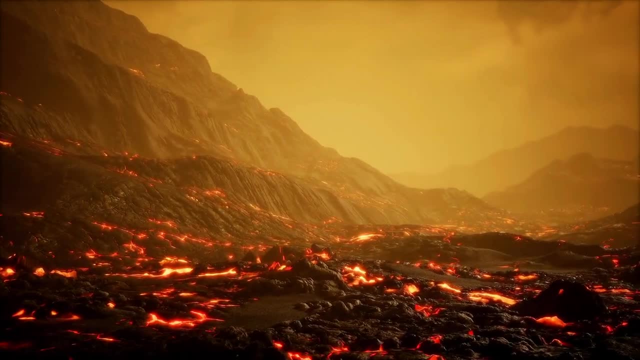 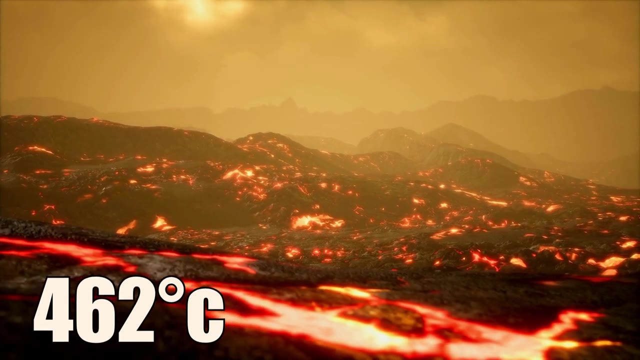 Venus is the second planet from the sun and the hottest planet in the solar system. It has a thick atmosphere of carbon dioxide and sulfuric acid that creates a runaway greenhouse effect. Because of this, the surface temperature is about 462 degrees Celsius, or 864 degrees Fahrenheit, and the atmospheric pressure is 92 degrees Fahrenheit. 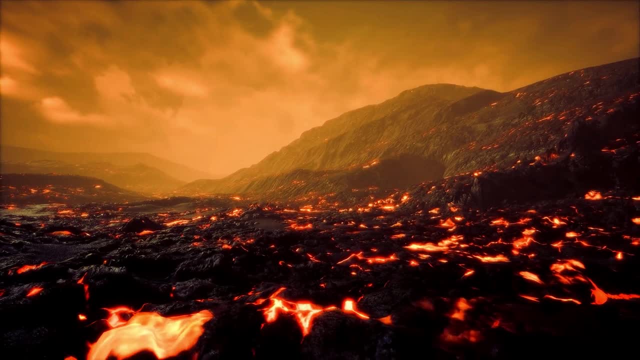 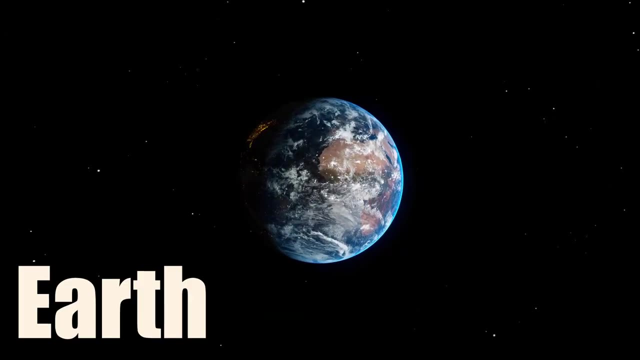 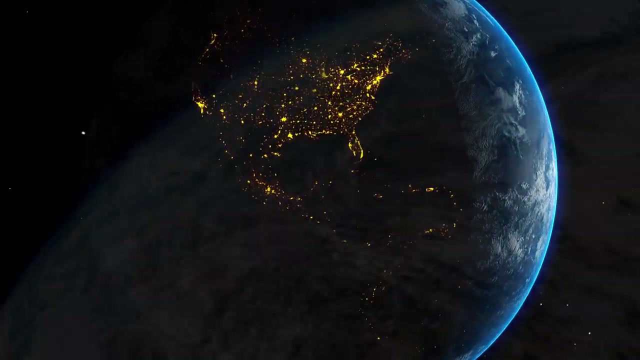 Venus has no moons and rotates very slowly in the opposite direction of most other planets. Earth is the third planet from the sun and the only known planet in the solar system that supports life. It has a moderate atmosphere of nitrogen and oxygen that protects it from harmful radiation. 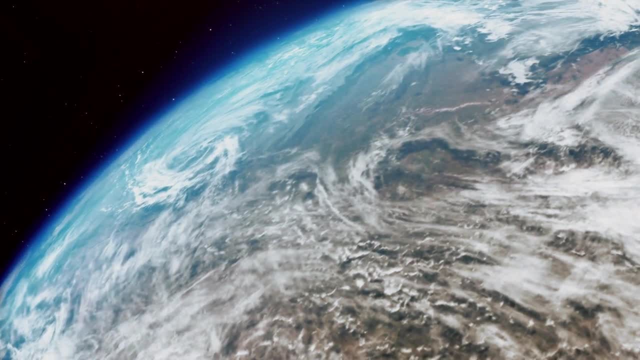 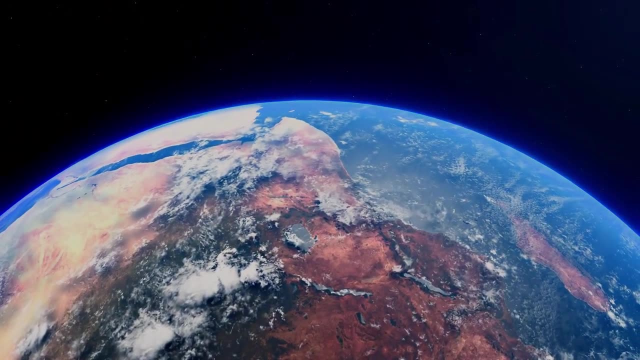 and allows for a stable climate. The surface is mostly covered by water, which makes up about 71% of the Earth's atmosphere. The surface is mostly covered by water, which makes up about 71% of the Earth's surface. Earth has one moon that influences its tides and seasons. 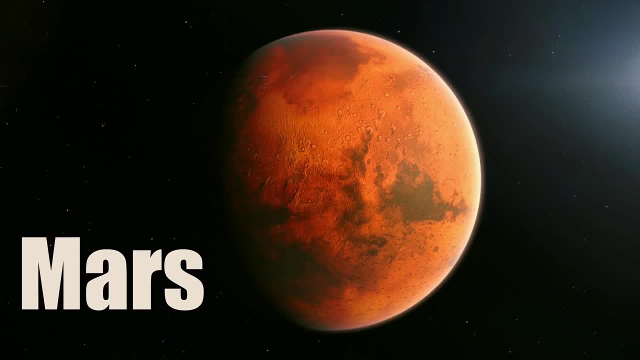 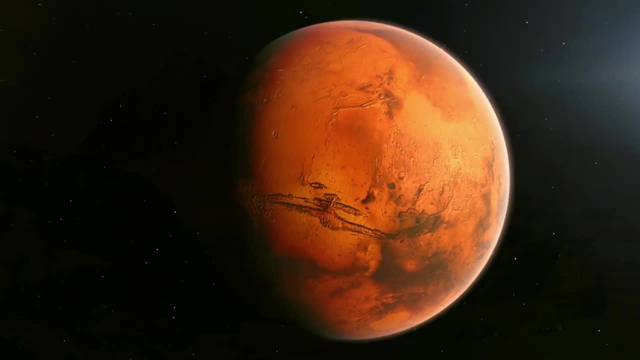 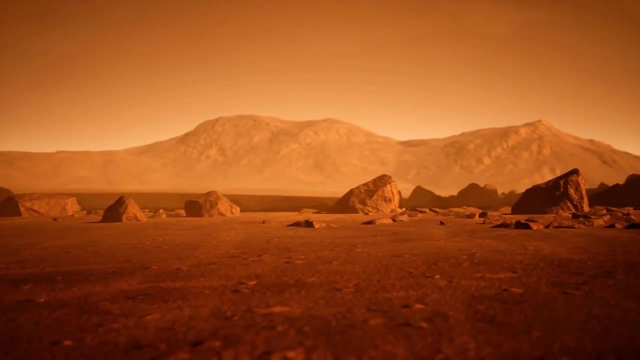 Mars is the fourth planet from the sun and the second smallest planet in the solar system. It has a thin atmosphere of carbon dioxide that allows for some weather phenomena such as dust, storms and clouds. The surface is mostly dry and rocky, with features such as volcanoes, canyons. craters and polar caps. Mars has two small moons of its own, and it is often considered a potential destination for human colonization because of its similarities to Earth. The second type of planet is the gas giant. These are the largest and most massive planets in our solar system: Jupiter, Saturn, Uranus and Neptune. 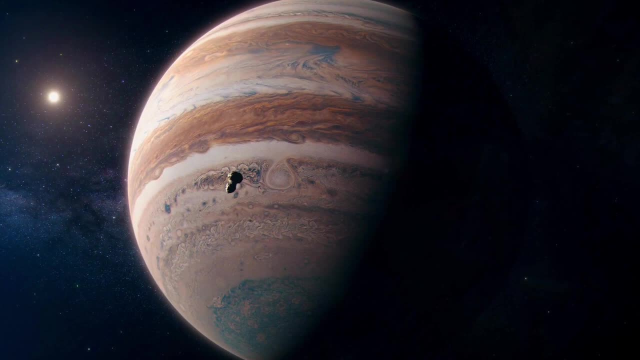 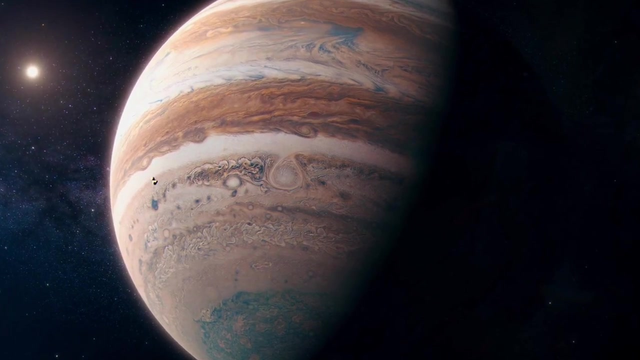 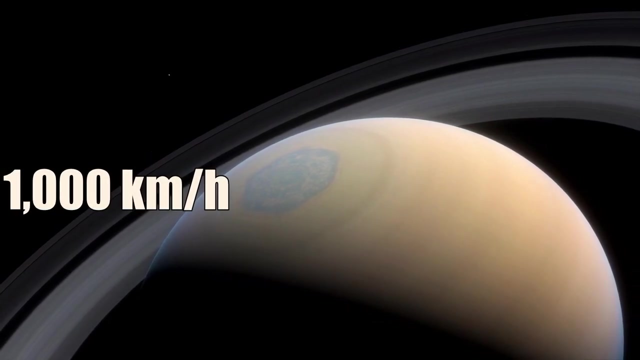 These planets have very large atmospheres and deep interiors of gas and liquid. They do not have a solid surface that we can stand on. Instead, they have layers of clouds, liquids, storms and winds that can reach speeds over 1,000 km per hour or 600 miles per hour. 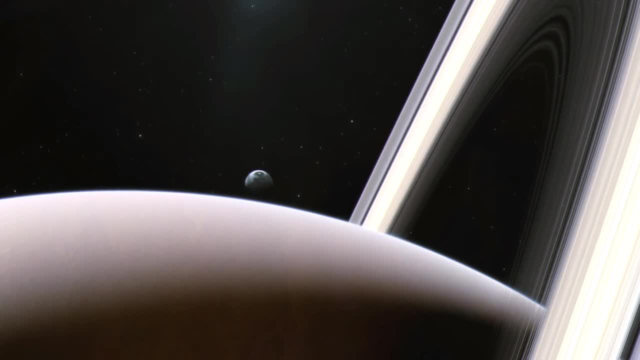 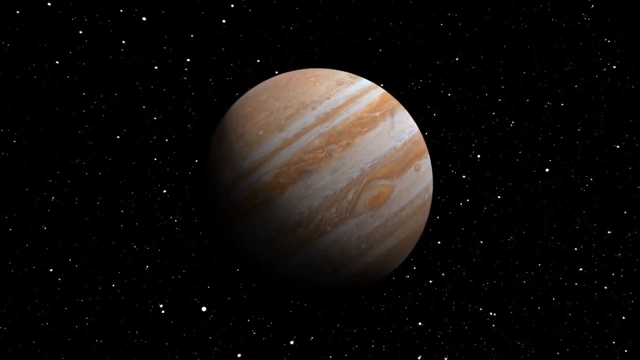 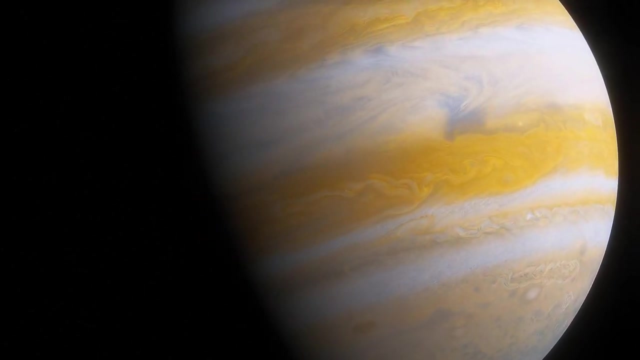 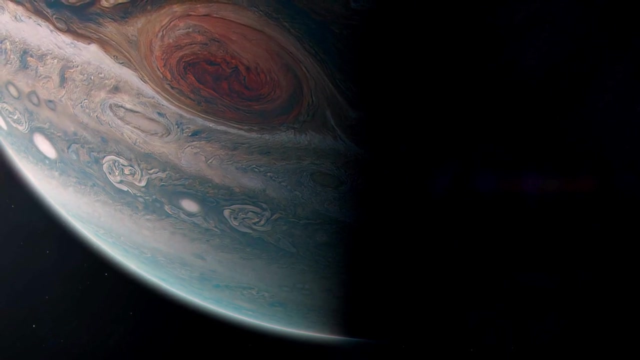 These planets also have many moons and rings that orbit around them. Mars is the fifth planet from the sun and the largest planet in our solar system. It has a thick atmosphere of hydrogen and helium that forms colorful bands and swirls. The most prominent feature on Jupiter is the Great Red Spot, a giant storm that has been 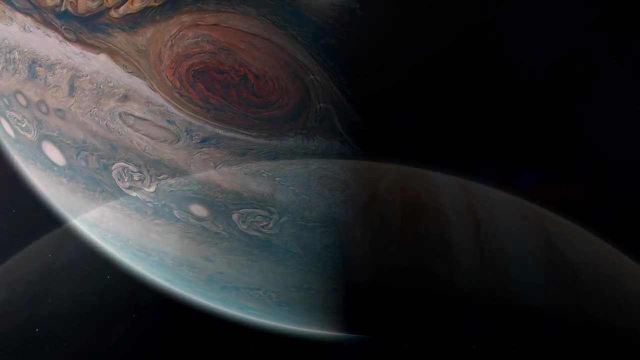 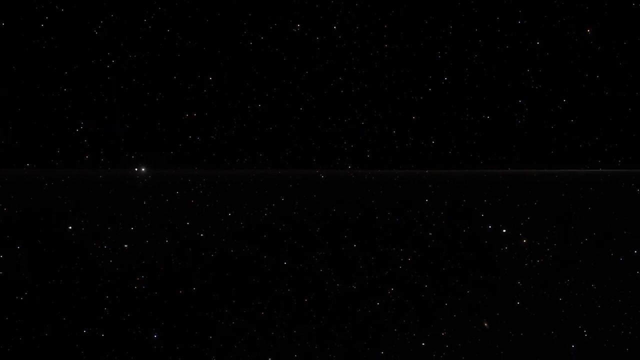 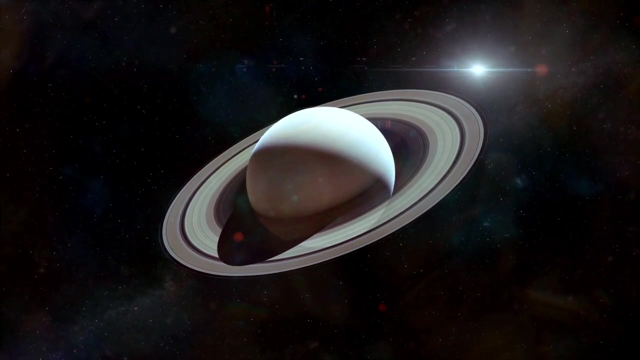 raging for centuries. Jupiter has at least 80 moons. Jupiter also has a faint ring system composed of dust particles. Saturn is the sixth planet from the sun and the second largest planet in the solar system. It has a similar atmosphere to Jupiter, but with more methane that gives it a yellowish hue. 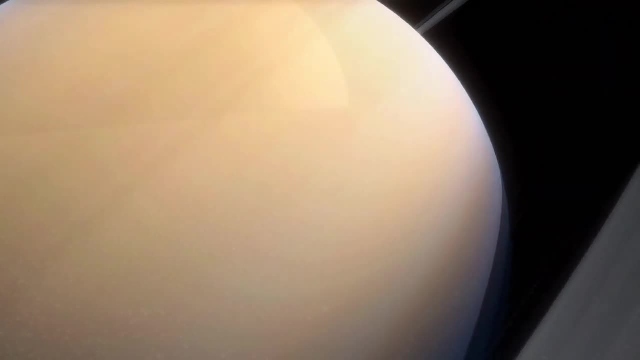 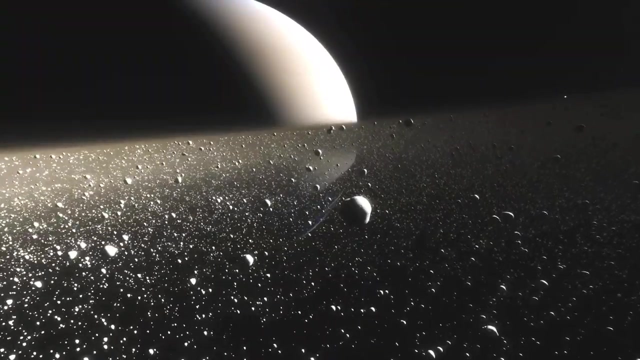 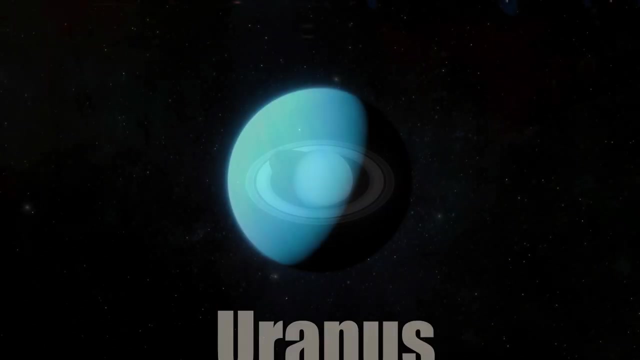 The most distinctive feature on Saturn is its magnificent ring system, which consists of billions of ice and rock particles that range in size from dust grains to mountains. Saturn has at least 145 moons. Uranus is the seventh planet from the sun and the third largest planet in the solar system. 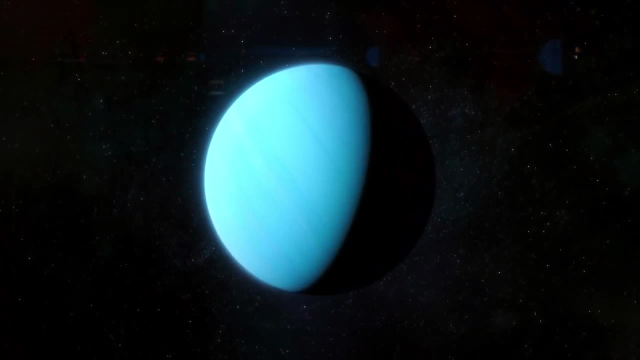 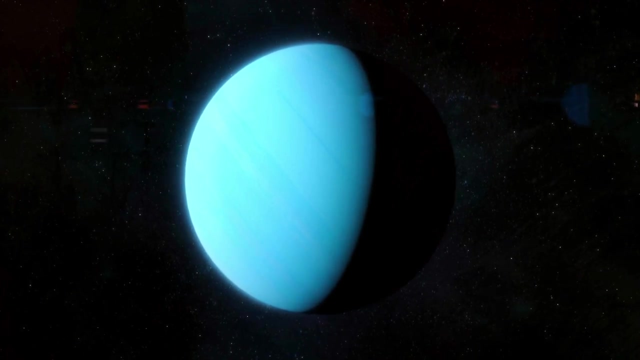 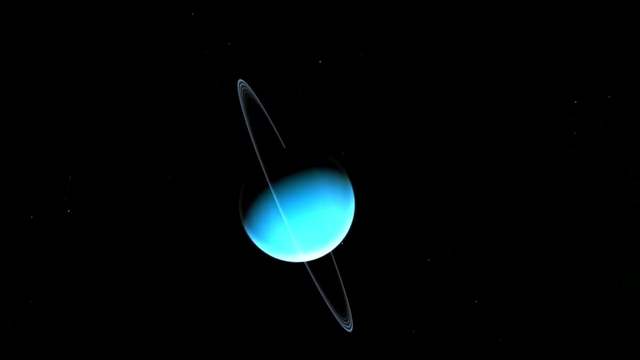 It has a thin atmosphere of hydrogen, helium and methane that gives it a bluish green color. Uranus is unique among the planets because it rotates on its side, with its axis tilted 98 degrees. This means that its seasons last for decades and its poles experience 42 years of daylight. 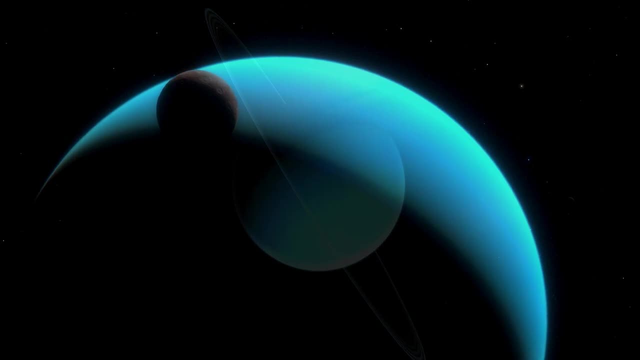 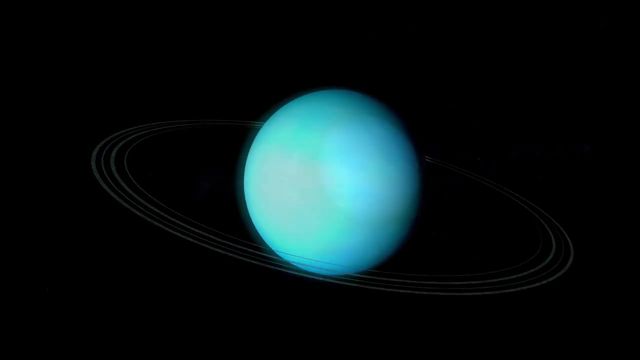 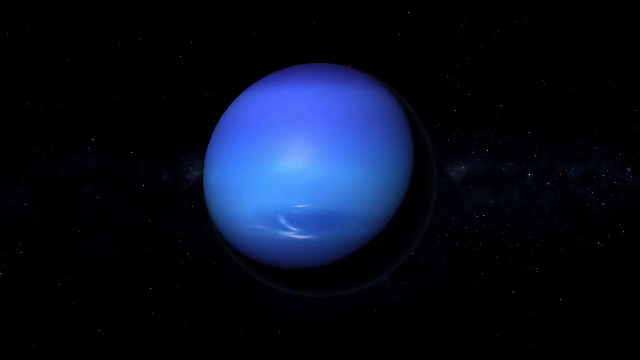 following the rise of the sun by 42 years of darkness. uranus has 27 moons and 13 rings that are also tilted. neptune is the eighth planet from the sun and the fourth largest planet in the solar system. it has a similar atmosphere to uranus, but with more methane that gives it a deeper blue color. 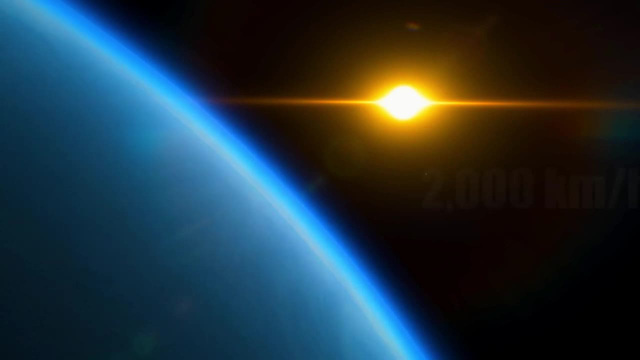 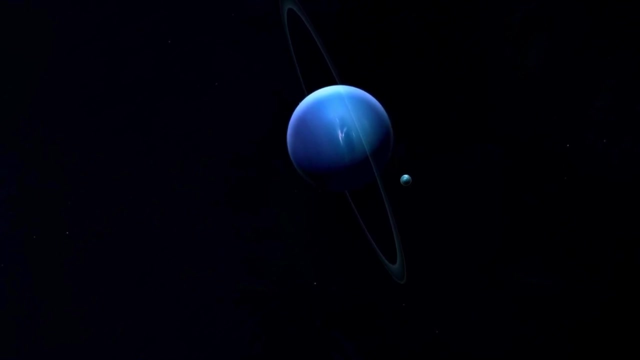 neptune is known for its supersonic winds that can reach speeds over 2 000 kilometers per hour or 1 200 miles per hour, making it the windiest planet in the solar system. neptune has 14 moons and six rings. one of its moons, triton, is the only large moon in the solar 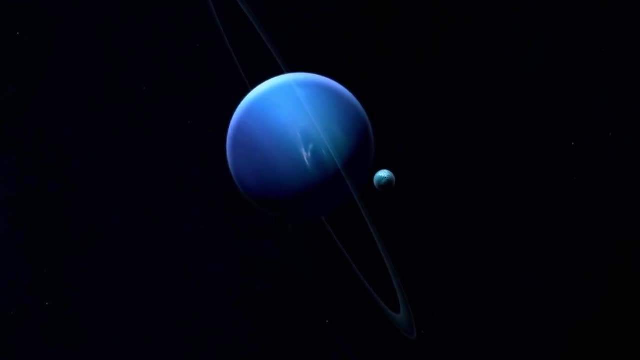 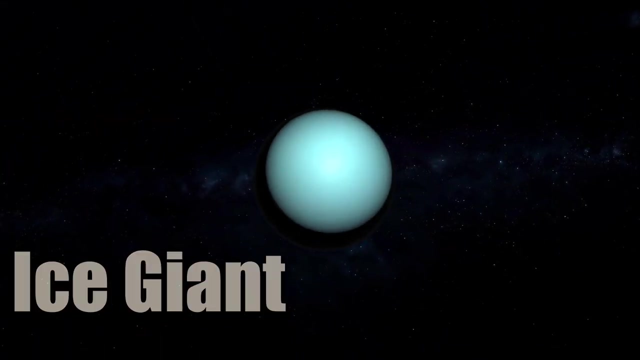 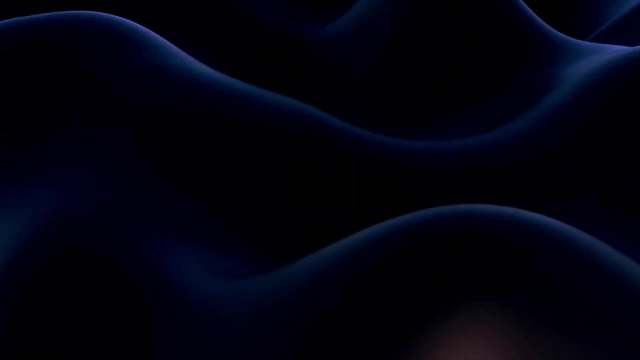 system that orbits in the opposite direction of its planet. the third type of planet is the ice giant. this is a subcategory of gas giants that includes uranus and neptune. these, These planets have a rocky core surrounded by a thick layer of water, ammonia and methane. 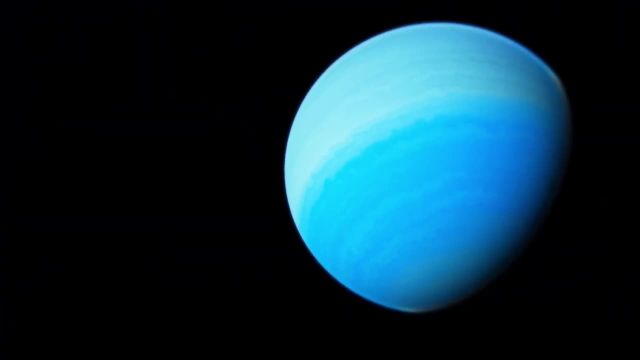 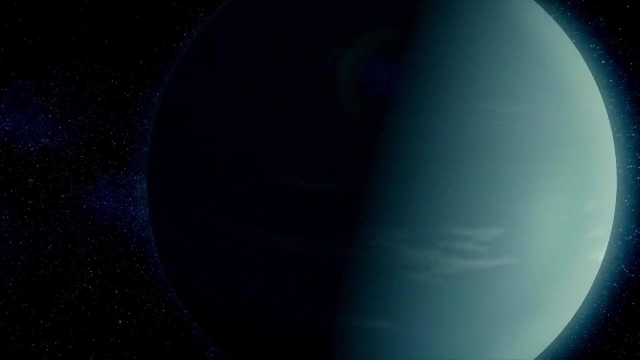 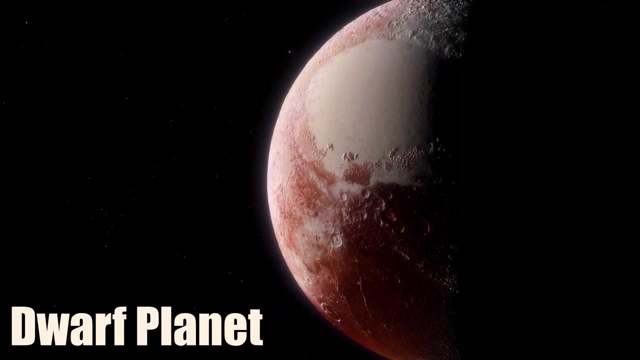 ices. These ices give them a bluish-green color and a lower temperature than the other gas giants. They also have strong magnetic fields that are tilted at a large angle from their rotation axis. The fourth type of planet is the dwarf planet. 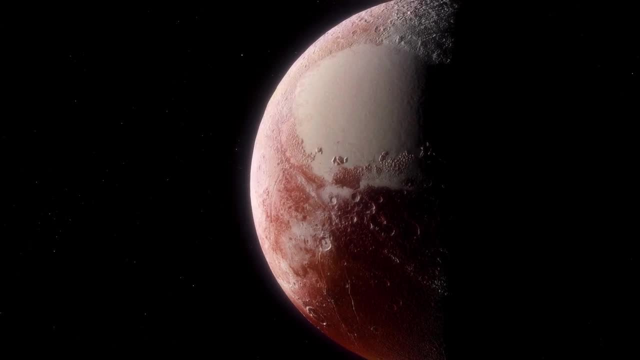 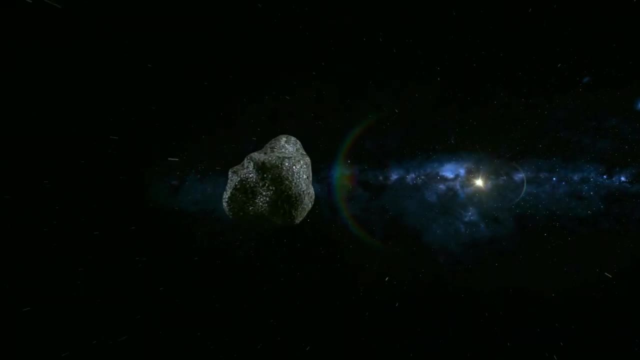 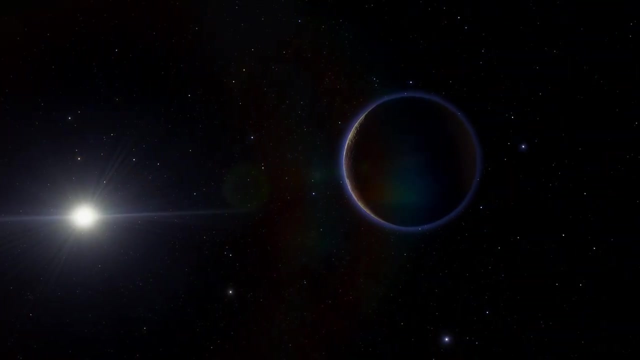 These are objects that share many characteristics with planets, but they are not large enough to clear their orbits of other debris. This means they share their orbit space with asteroids, comets and other small bodies. There are five officially recognized dwarf planets in our solar system. 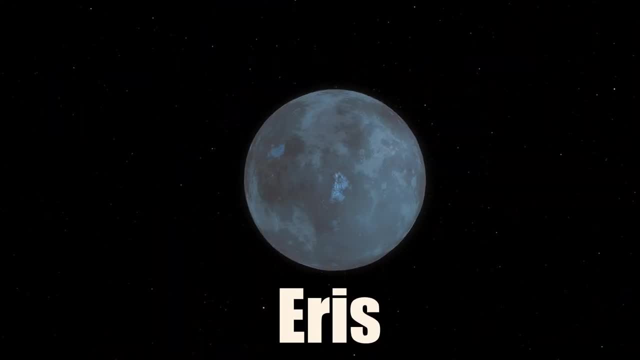 Pluto, Cirrus, Eris, Haumea and Makemake. These objects are known as dwarf planets because they are large enough to clear their orbits of other debris. These are objects that share many characteristics with planets, but they are not large enough. 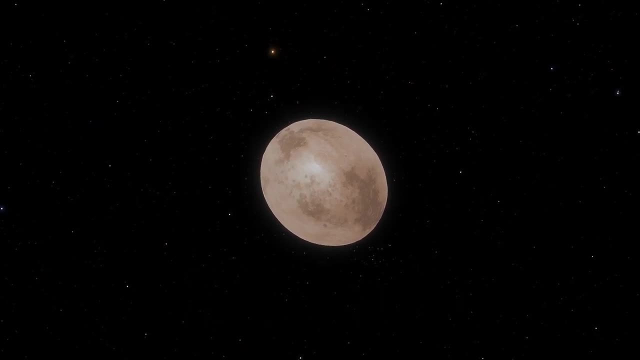 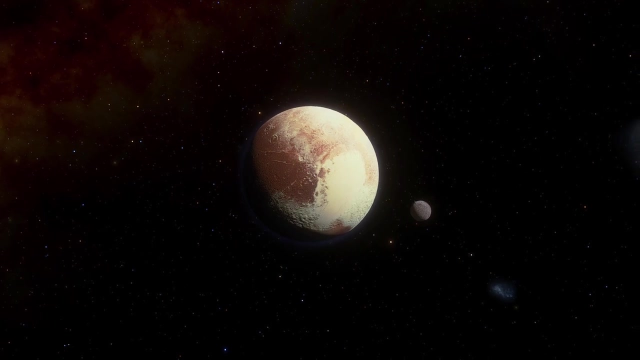 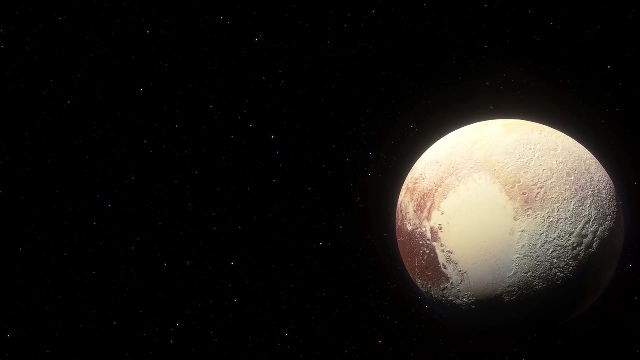 to clear their orbits of other debris. These objects are very diverse in size, shape, composition and orbit. Some of them even have moons of their own. Pluto is the largest and most famous dwarf planet in the solar system. It was once considered the ninth planet until it was reclassified in 2006.. 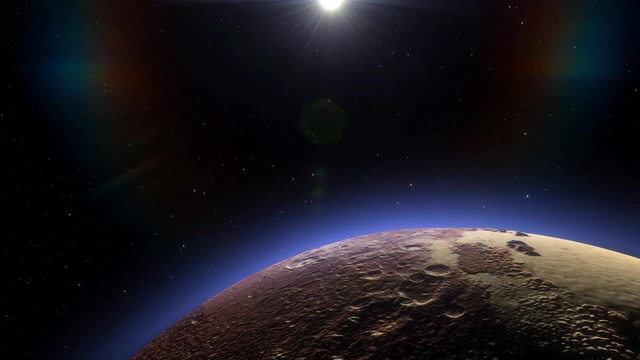 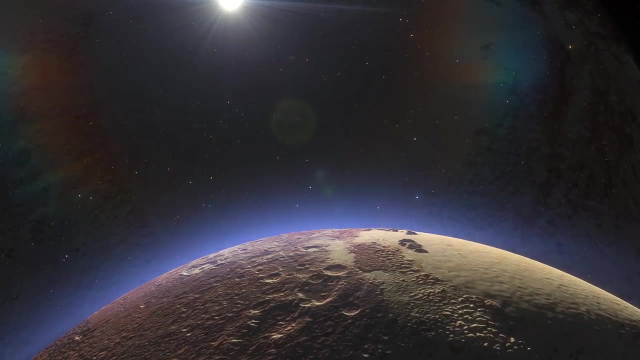 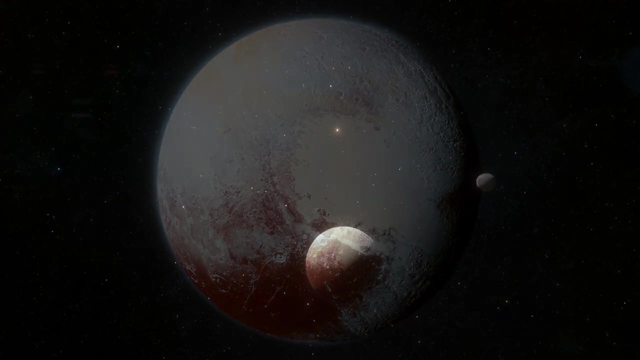 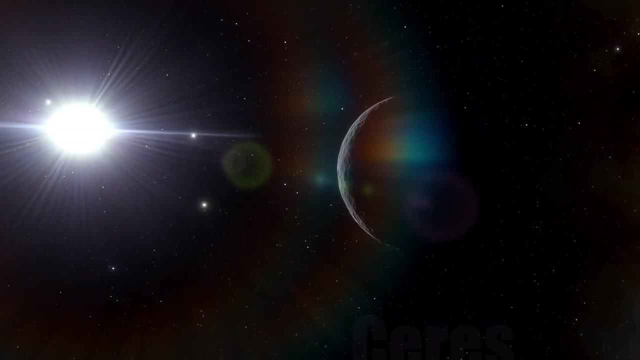 Pluto has a thin atmosphere of nitrogen, methane and carbon monoxide. It freezes and sublimates depending on its distance from the Sun. The surface is mostly covered by ice and has a large heart-shaped region. Pluto has five moons, including one large one called Charon that is almost half its size. 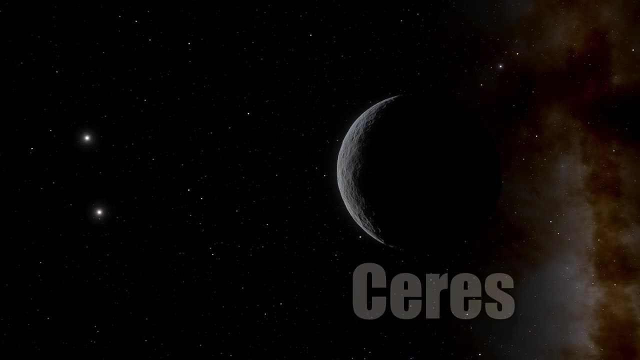 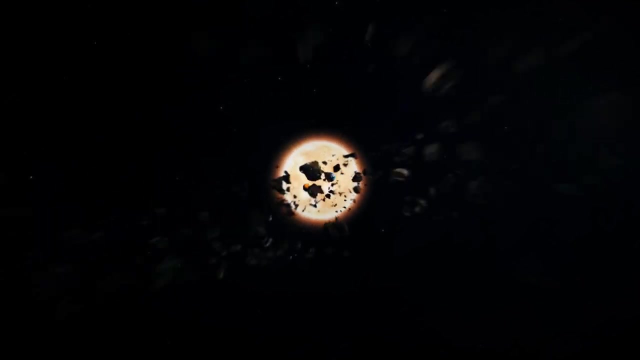 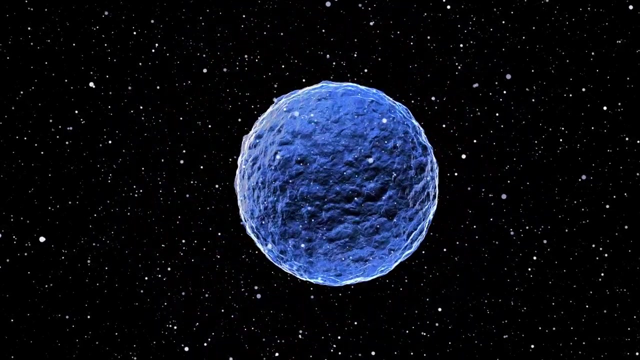 Cirrus is the smallest and closest dwarf planet to the Sun. It is also the largest and most massive object in the asteroid belt between Mars and Jupiter. Cirrus has a rocky core and a thick mantle of water ice that may contain an underground ocean. 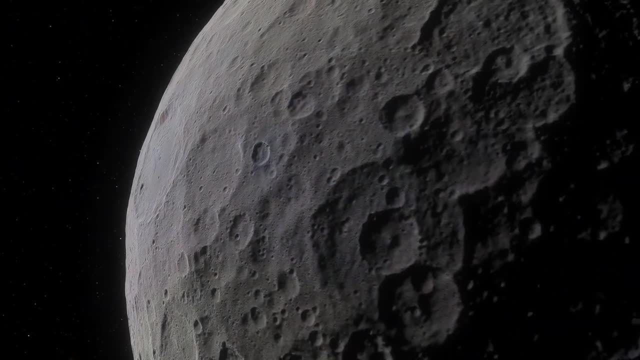 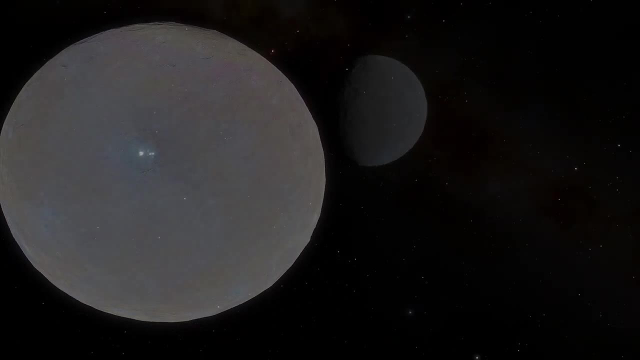 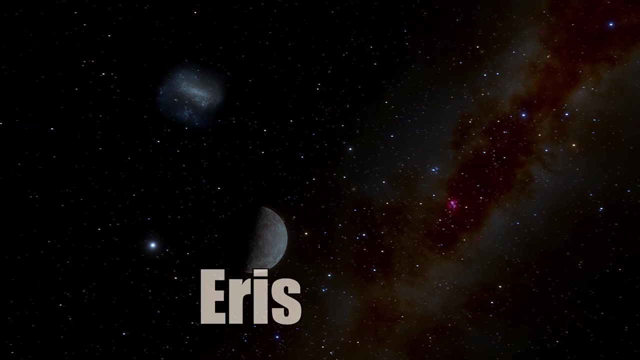 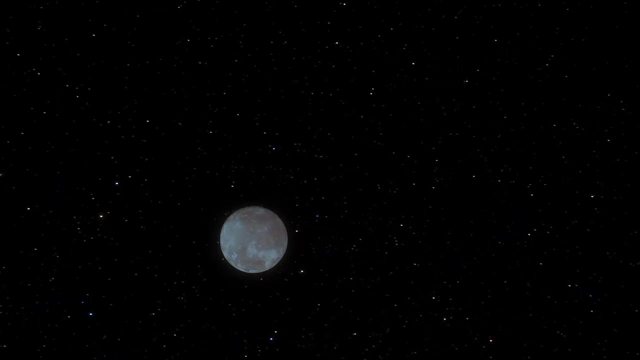 The surface is mostly dark and cratered, but has some bright spots that may be salt deposits or ice volcanoes. Cirrus has no moons. Eris is the most distant and second largest dwarf planet in the solar system. It is also the most massive dwarf planet, slightly heavier than Pluto.